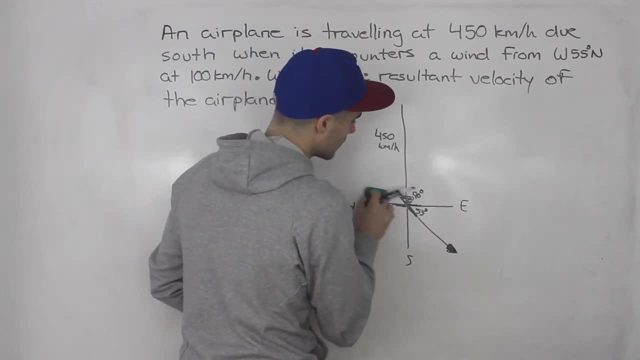 erase this other one, so there's just less going on here, not to confuse you. so got the plane, you got the wind, and so we've now got an angle which will be at 45 degree south, north east of west, 55 degrees north west, 55 degrees north east of east. 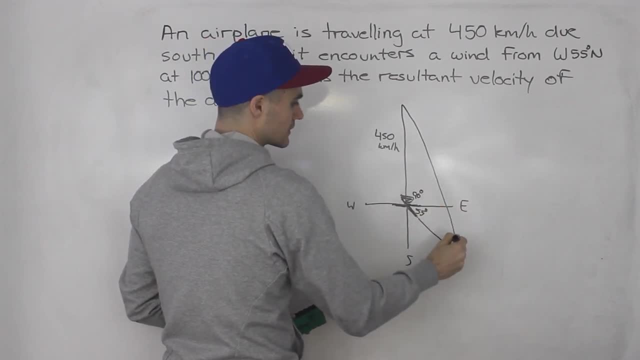 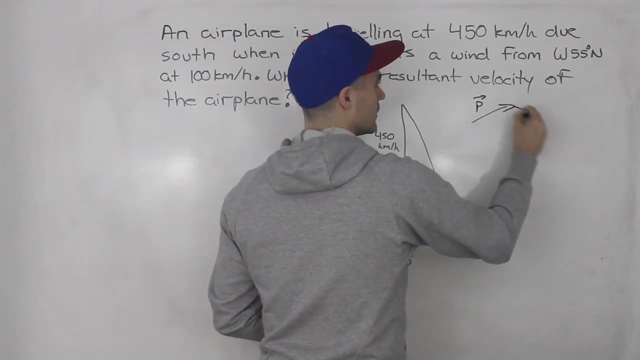 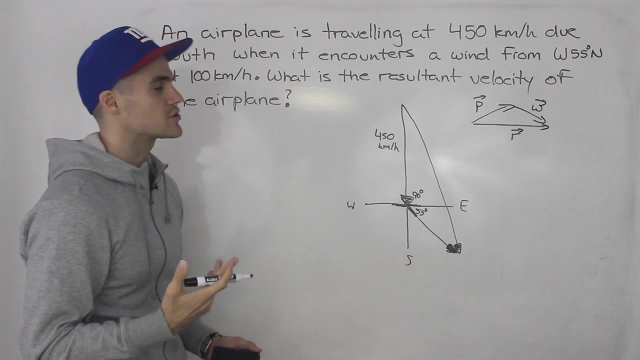 So the resultant is going to look like that, going that way, right? Because you have a plane vector, you got a wind vector and then you have a resultant vector, right? So with these types of questions, always be aware of what they are giving you and what. 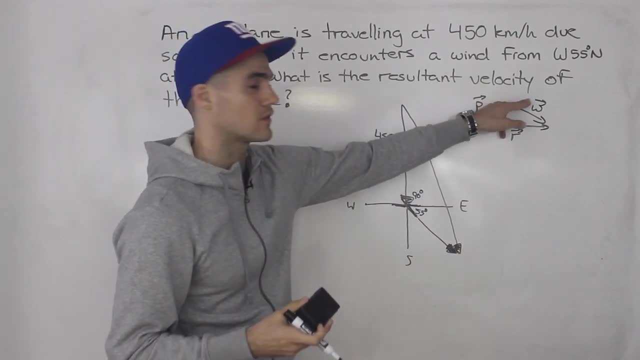 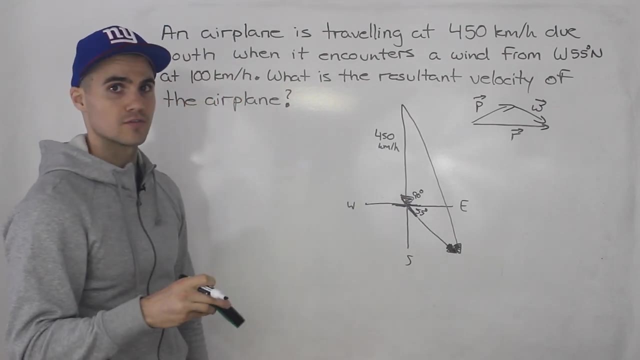 you're being asked In this case, we're simply given the plane vector, we're given the wind vector, we're asked for the resultant vector, the resultant velocity. But, as you saw in the lecture videos which I highly recommend you going over because 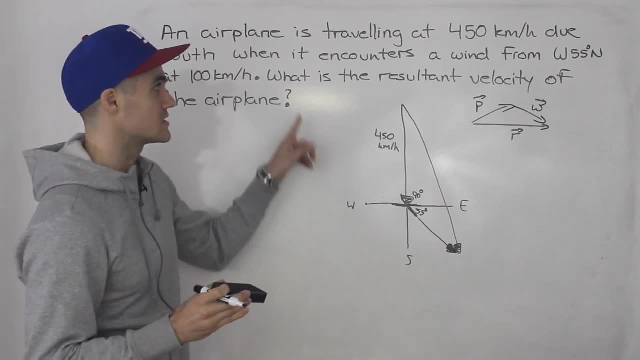 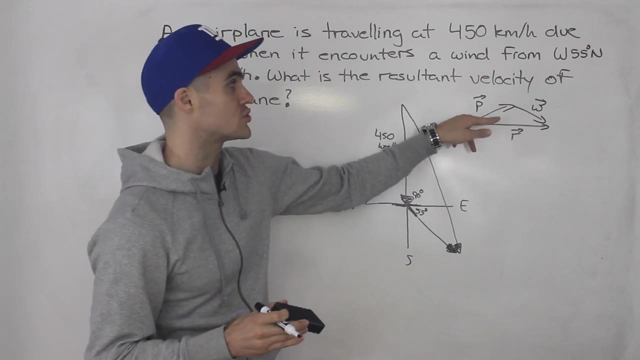 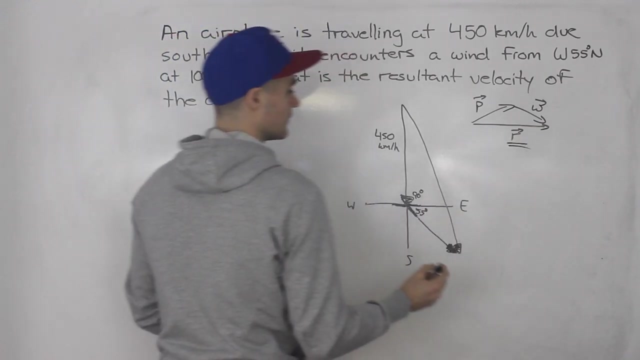 I go through a lot of tough questions in the lecture videos dealing with airplanes and winds. sometimes you're asked for different things. Sometimes you're asked for the wind velocity or the wind direction, or which direction does the plane have to fly right? But in this case we're just simply asked for the resultant. 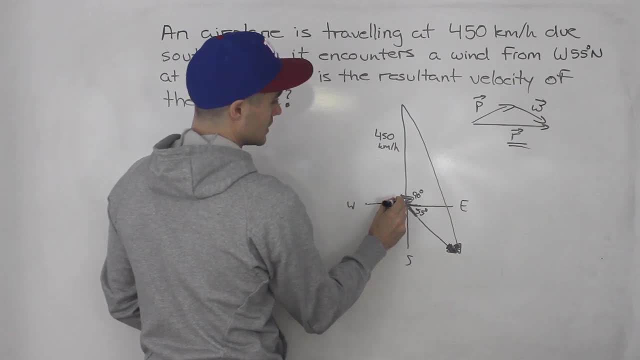 So we got the plane going south. then we got the wind coming from west- 55 degrees, So that's the same as going towards east, 55 degrees south, And then the resultant is going to be here, right, And then the wind has a speed of 100 kilometers per hour. 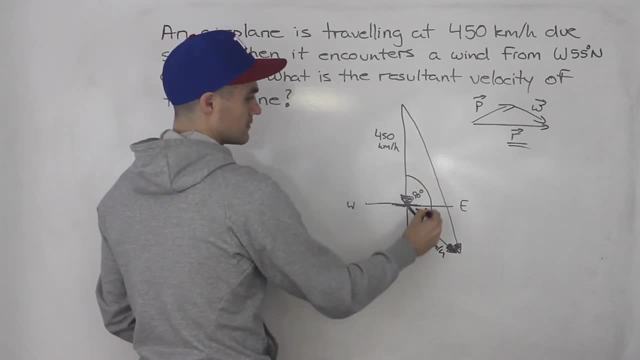 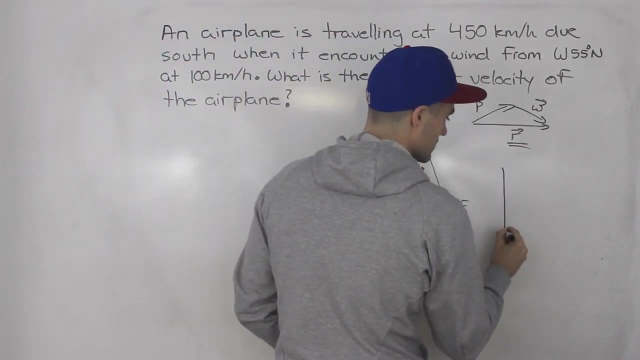 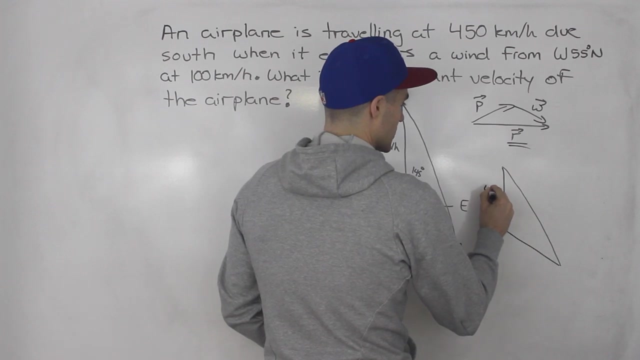 So notice that we just got a triangle. now We can add these two angles, So 90 plus 55, that's 145 degrees. Let's actually draw this triangle down here again a little nicer. So this is 450,, this is 100, and then this is 145 degrees, right? 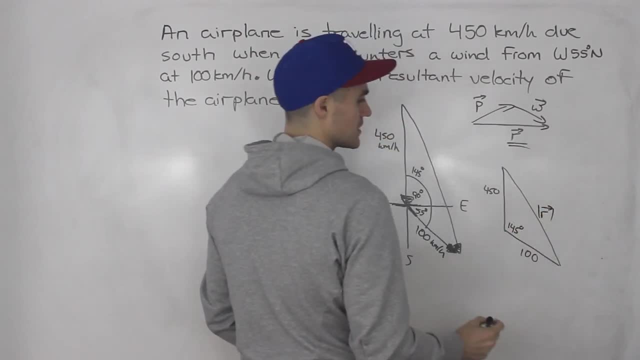 And we're looking for this resultant. So that's like the speed of the resultant And then the direction we're going to solve for this data here, right? So let's start off by solving for that resultant speed. So to do that, we would do cosine law. 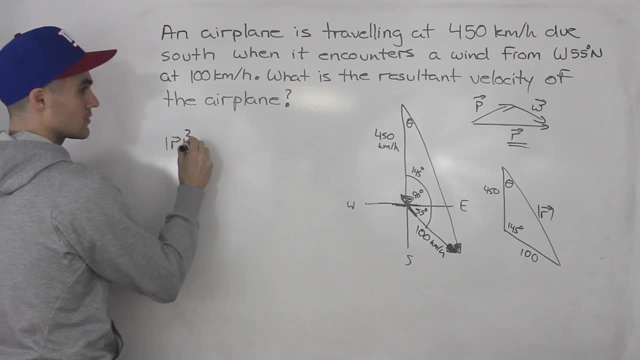 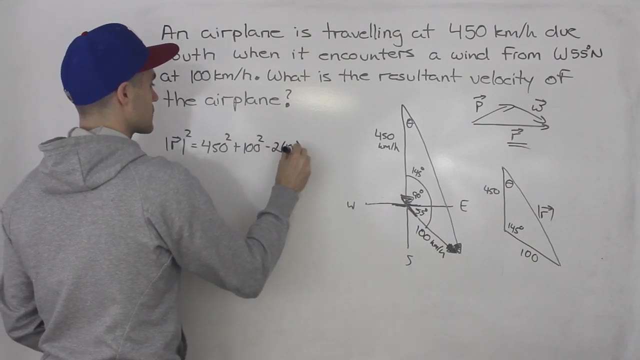 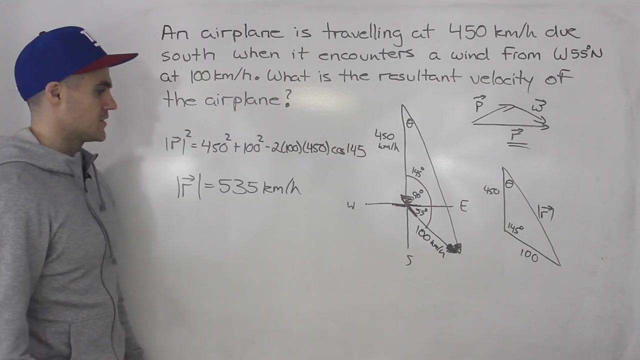 So we got the resultant: squared E Equals 450 squared plus 100, squared minus 2 times 100 times 450 times cos of 145.. So when you do that in the calculator you end up getting 535 kilometers per hour. 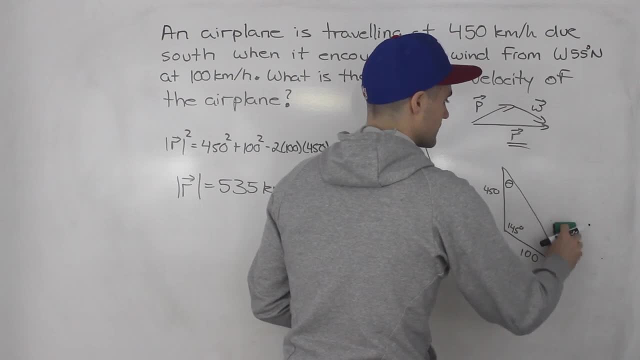 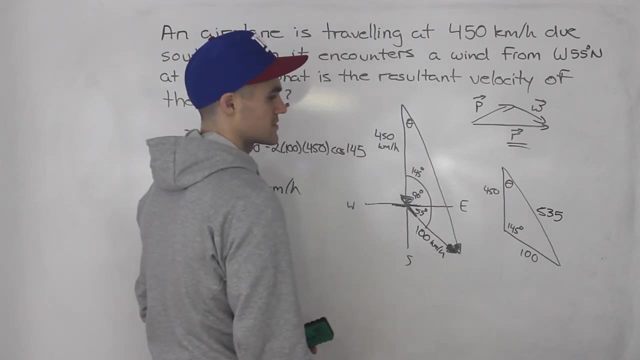 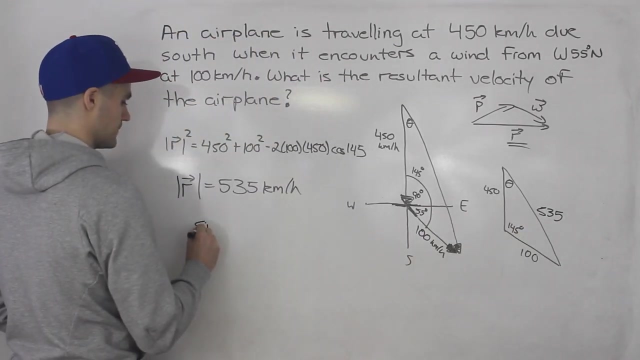 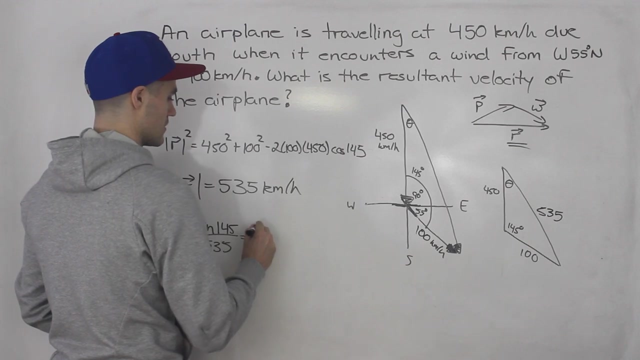 So that there is the resultant speed. But they want the resultant velocity. So we're also going to have to get the direction. So we're going to solve for this theta, Solve for that theta. We can use sine law. So we could do: sine of 145 over 535 equals sine of theta over that opposite side, 100. 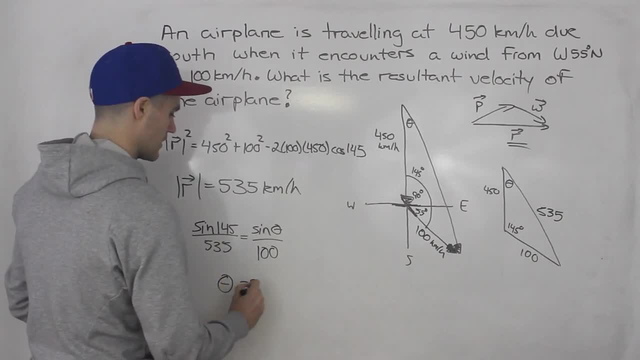 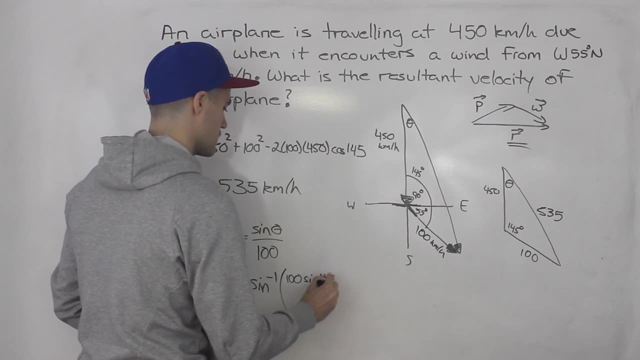 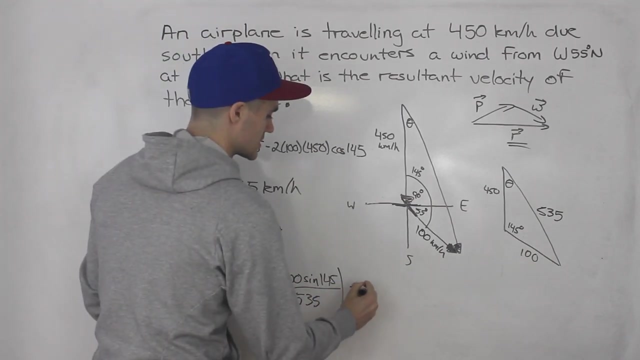 Okay, and then when we cross multiply, when we isolate for that theta, we'll basically be taking the inverse of 100 times sine of 145. So we're going to have to solve for that theta All over 535.. And when you do that in your calculator you end up getting 6.15 degrees. 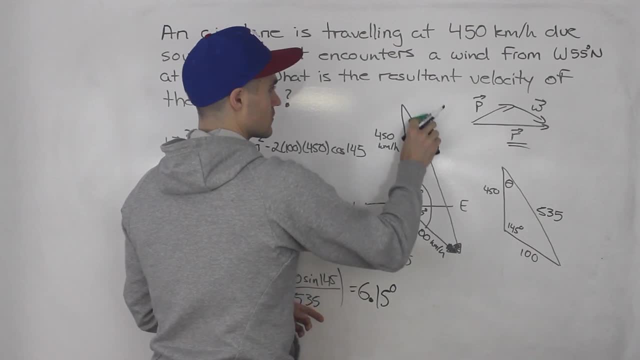 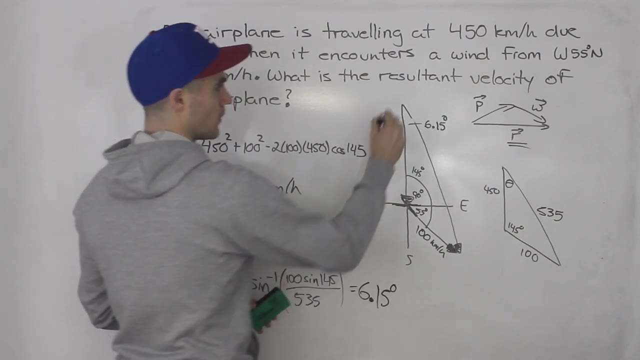 So that there is 6.15 degrees, And then maybe let's write that angle here: 6.15 degrees. So how can we state that as a direction? Well, if we draw a compass here, we got north, east, west. 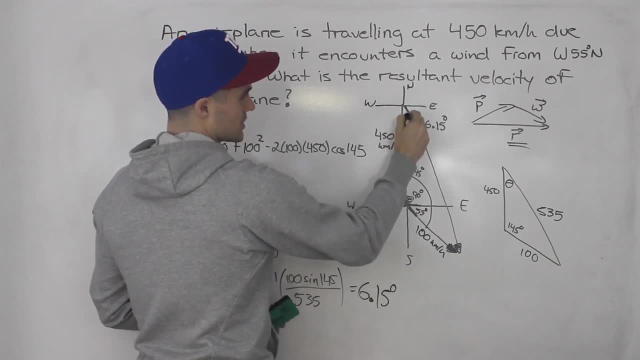 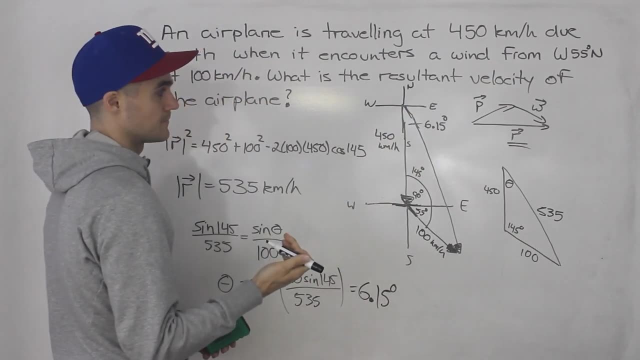 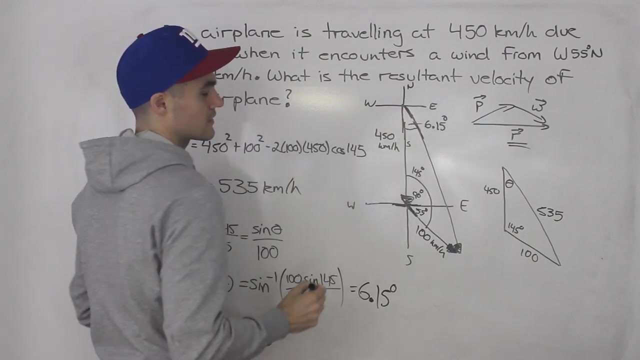 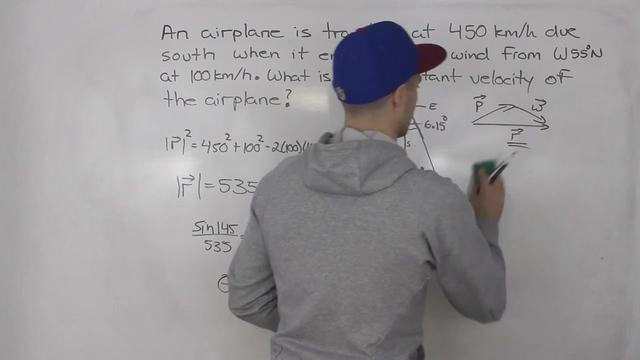 then this is going south. so this direction here is going to be what? South 6.15 degrees towards the east, South 6.15 degrees towards the east for the direction of this vector here. So the final answer for this question: the resultant velocity is the speed, so 535 kilometers per. 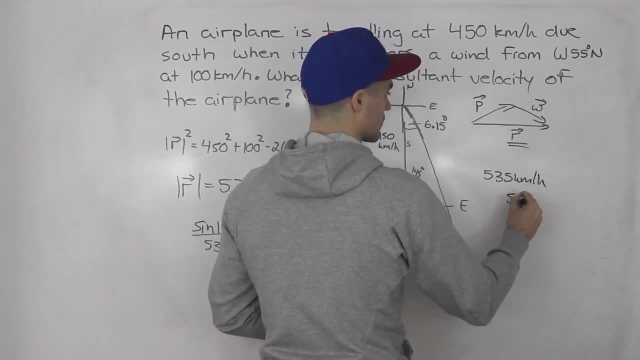 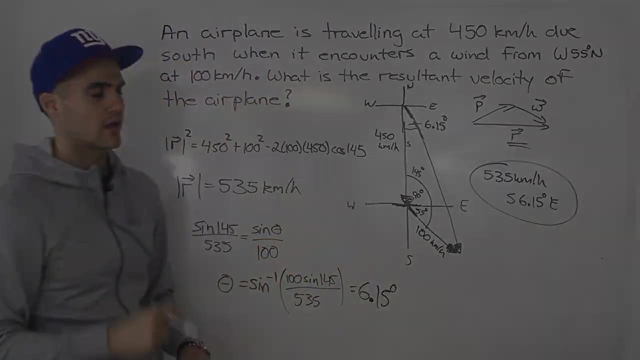 hour in a direction south, 6.15 degrees east. That there is the final answer.